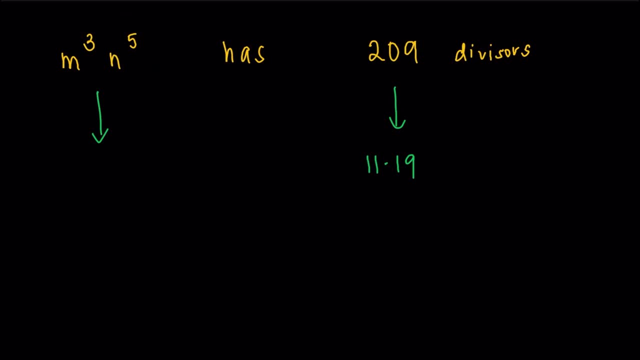 prime factorization of that. it's going to be something like this: It's going to be A raised to 10, then B raised to 18, something like that. Now, obviously there is another possibility where 209 comes from C raised to 208, a certain prime number raised to 208.. By the way, A, B, C are prime numbers. 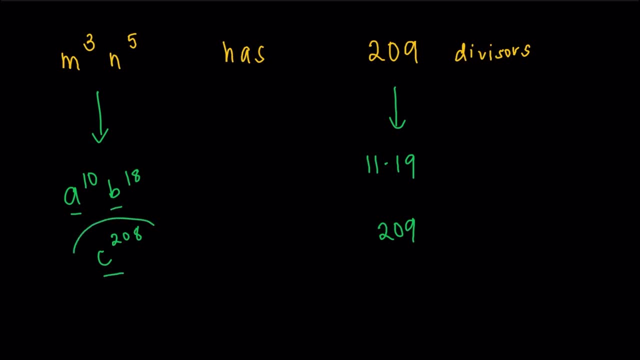 I said it's going to be a prime factorization But well, C raised to 208 is impossible because well, M and N are relatively prime so they can't be the same prime number. So it's going to be probably the 11 times 19 case. So M cubed N to the 5th should look something like: 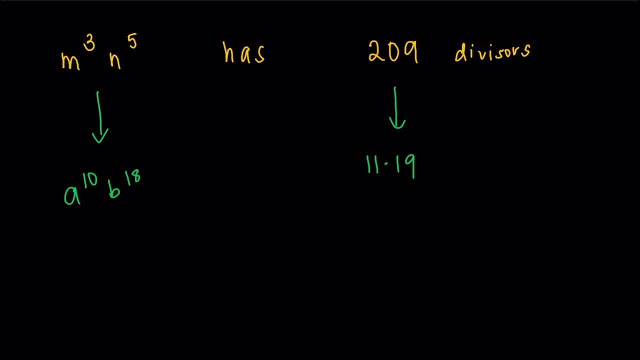 this Now. I think it's rather interesting here that 10 is divisible by 5 and 18 is divisible by 4.. Well, in fact, that's going to be the motivation for us to do Well M I could. 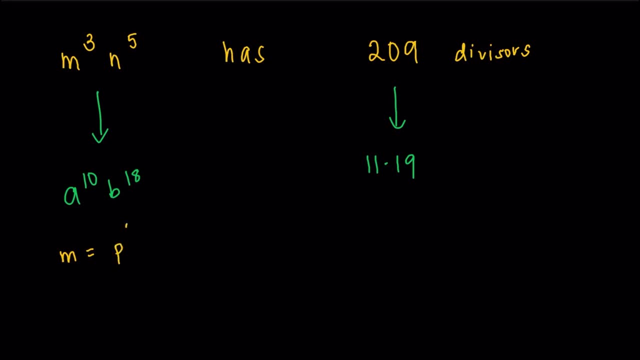 write M as a certain prime number, P raised to 6, because well, 3 times 6 is going to give 18, and then 5 times 2 is going to give us 10.. So I think I'm motivated to put N as. 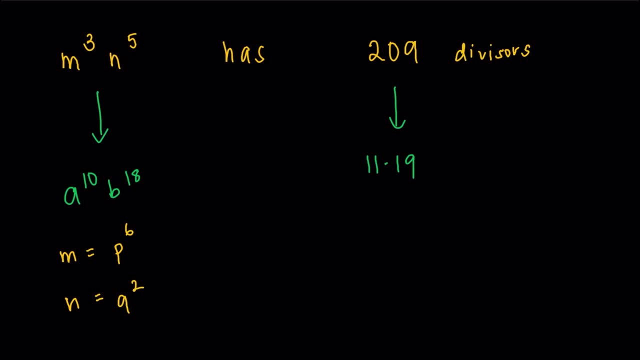 Q squared. Now I could also try actual values of P and Q, if you guys are a little bit paranoid about me using variables here. So if M equals 2 raised to 6.. And N equals 3 squared, well, M cubed N to the 5th is essentially going to become 2 raised. 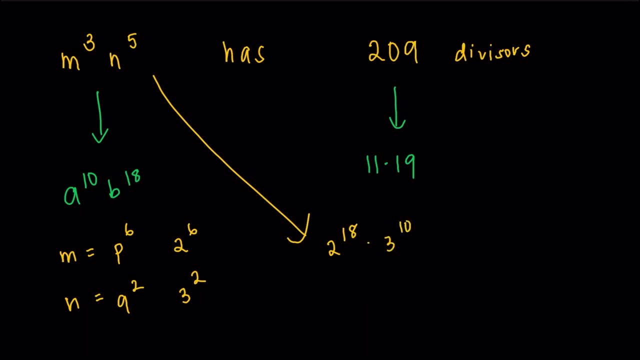 to 18 times 3, raised to 10.. That's in a prime factorization. That's good. Taking the exponents, adding 1 to it, 19 and 11, and there we go: 209 it is. So, whether you're the technical, 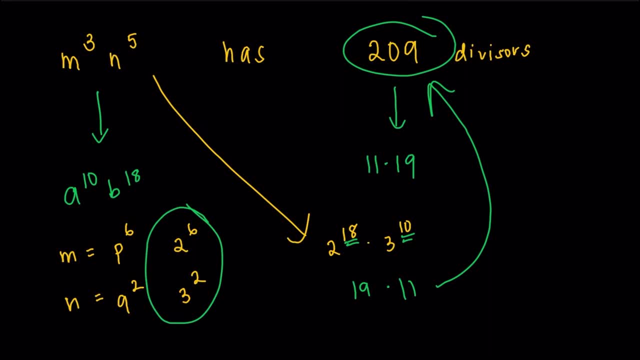 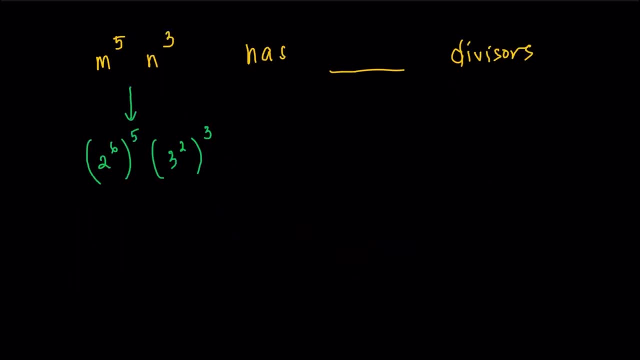 to use the 2 raised to 6 and 3 squared. So I'm just going to use the 2 raised to 6 and 3 squared And check how many positive divisors does M to the 5th times N cubed have. So 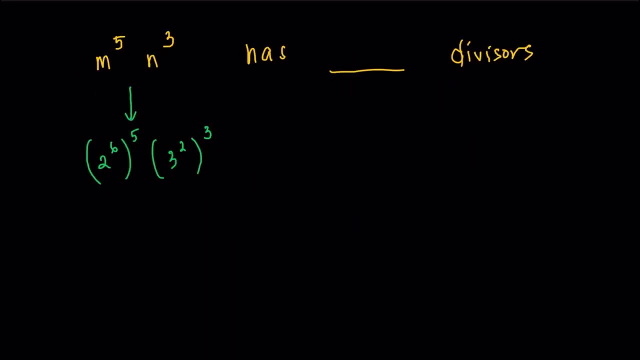 2 to the 6 is M, 3 squared is N. Just directly substitute it in Use the laws of exponents. That's going to be 2 raised to 30 times 3 raised to 6.. We already have the prime factorization.